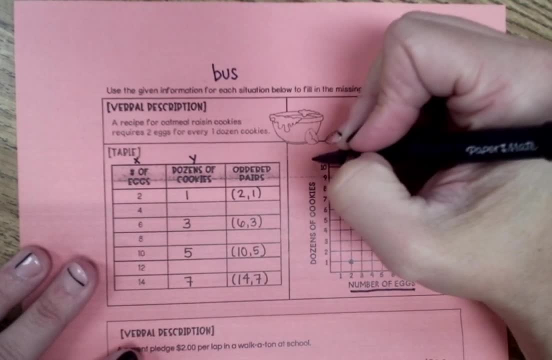 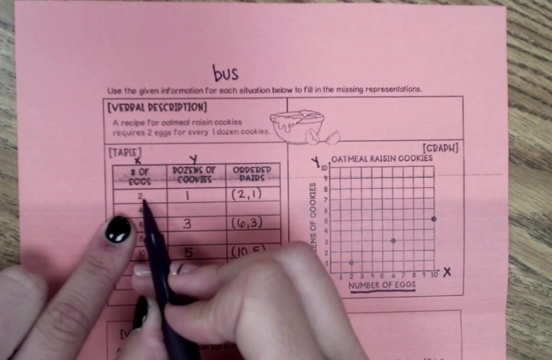 of eggs was there And then dozens of cookies is over here on our y axis. So that's how I knew that that was my y value. So again, if I look at this every time, I know that I'm just going from two to 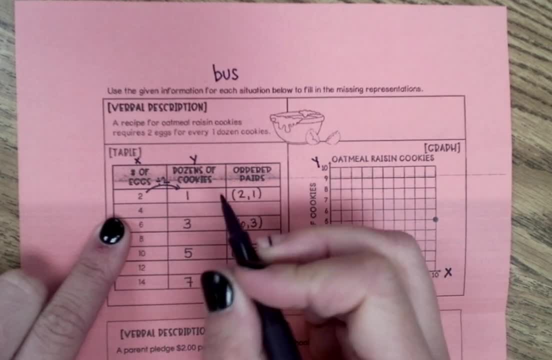 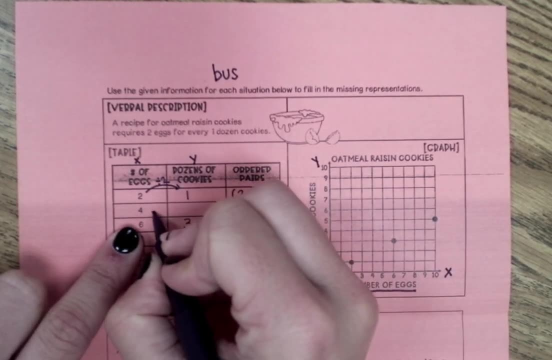 one, I had to divide By two, So that's my rule. I'm dividing by two every time on here to figure out how many dozens of cookies I will have. So four divided by two gives me two. So my ordered pair here would be: 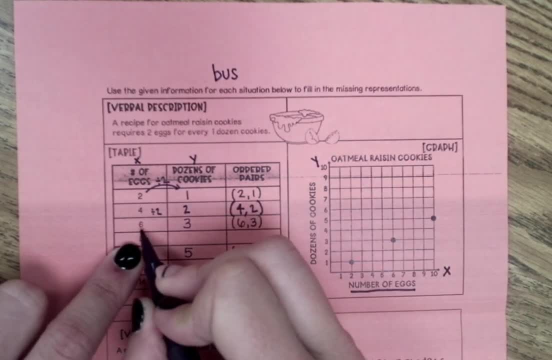 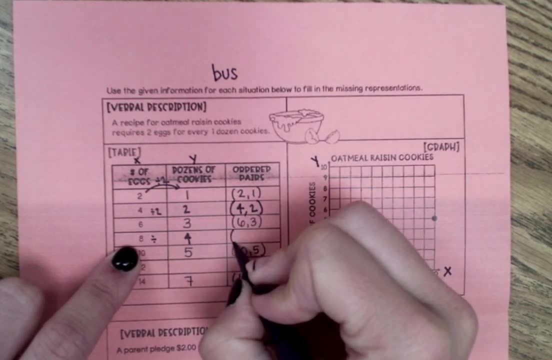 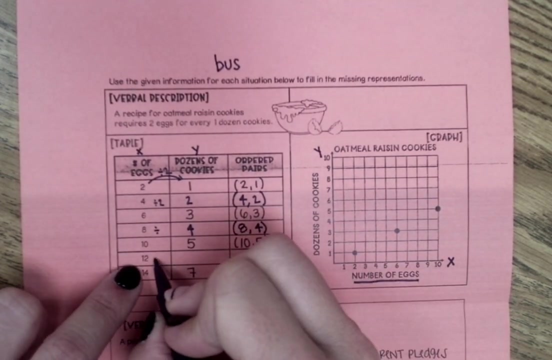 four comma two. Six divided by two does equal three, So that checks out. Eight divided by two is four, So my ordered pair here is eight comma four. 10 divided by five does equal five, So that checks out. So we're going to do two, And then we're going to divide by two, So that checks out. 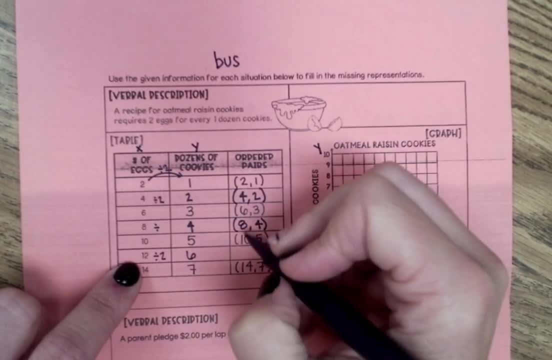 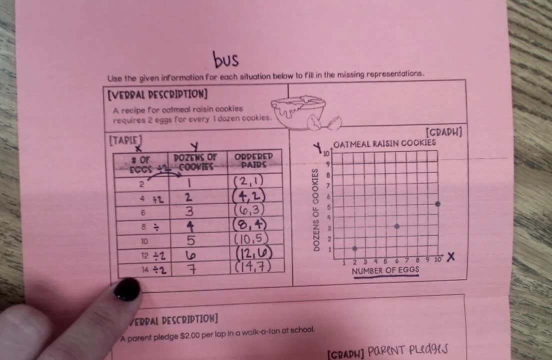 12 divided by two, That gives me six. So my ordered pair here is 12 comma six, And then we'll just check again. 14 divided by two does equal seven, And then we can see it there. So now we're. 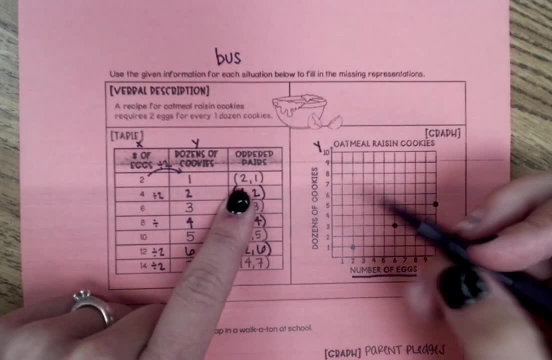 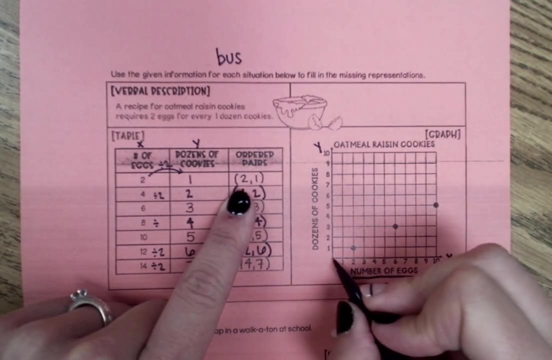 going to plot these points here And it looks like we've kind of started it for you. So we know our first ordered pair. we're going to start at our origin: zero, zero. right here. We're just working in quadrant one for these. So right here is our zero, zero origin. So you're always going to start. 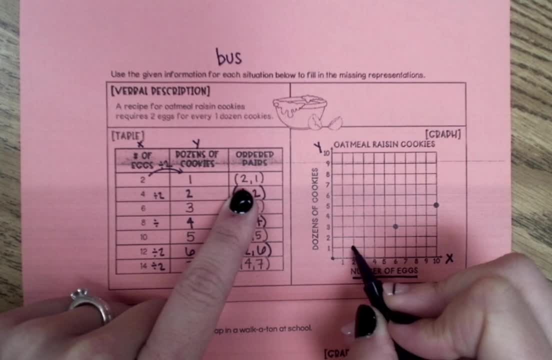 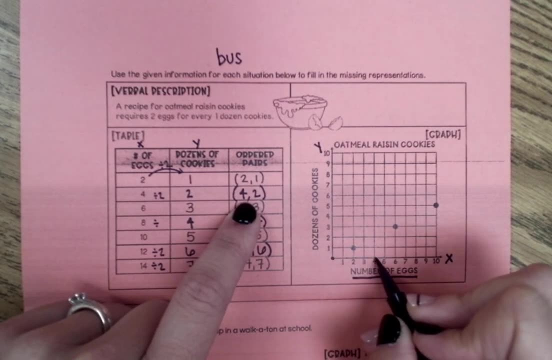 here. So we go over two up one. It's already plotted with a dot. Now we're going to go back to our origin And we're going to plot the point four, comma two. So we go over four up two. plot with a dot. Over six up three was done. 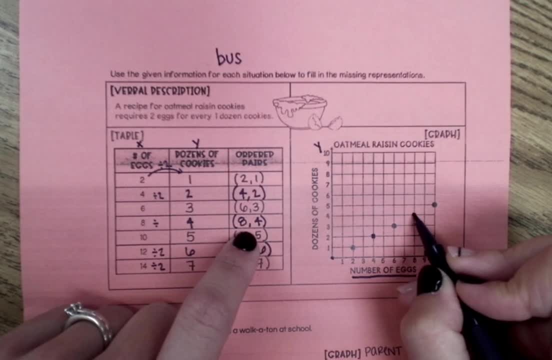 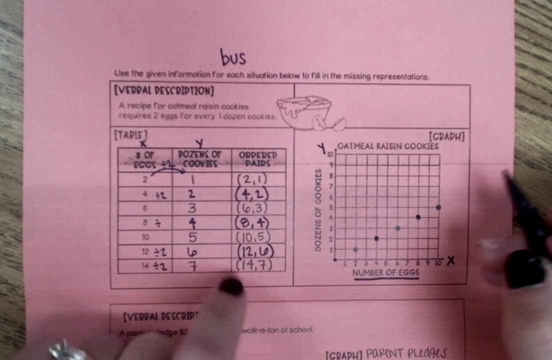 for us. So we're going to go over eight, up four- plot with a dot, Over 10, up five- plot with a dot, And then the last two points are actually off of our graph, So we can connect those points. 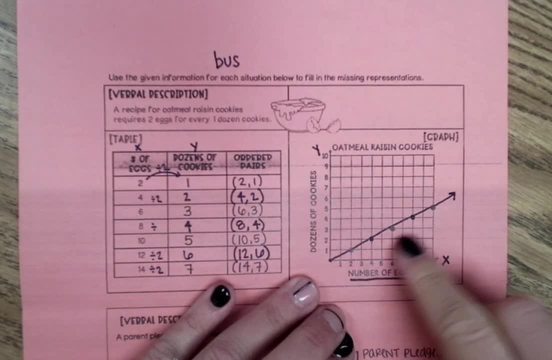 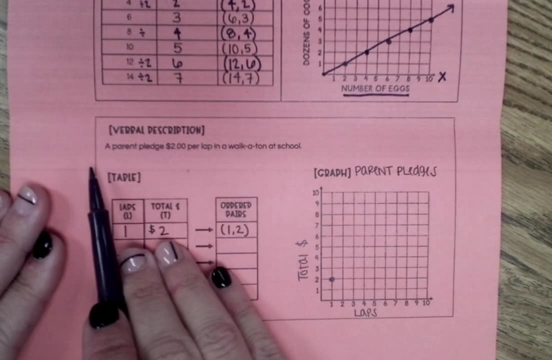 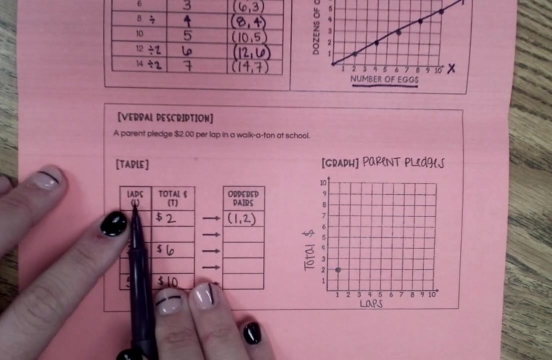 and extend it out with a little arrow to say it's going to continue on. All right, let's look at our next one. This is a parent pledge. A parent pledges $2 per lap in a walkathon at school. So here's our table. We have laps which are down here at the bottom, So we 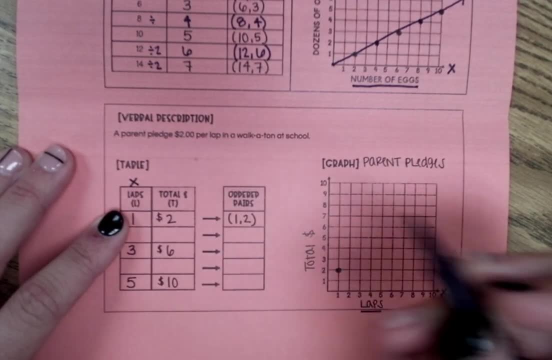 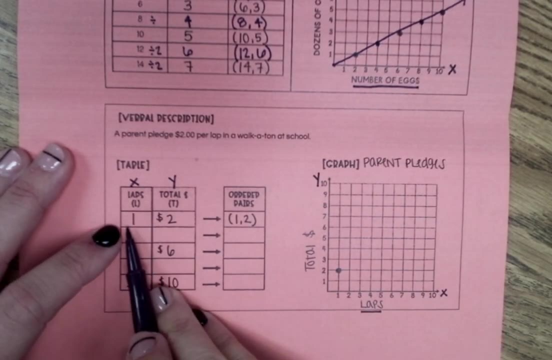 know that this is my x value because it's on my x axis And we have total money which is over here on the side. So that's my y value because it's on my y axis. So for every one lap it's $2.. So we 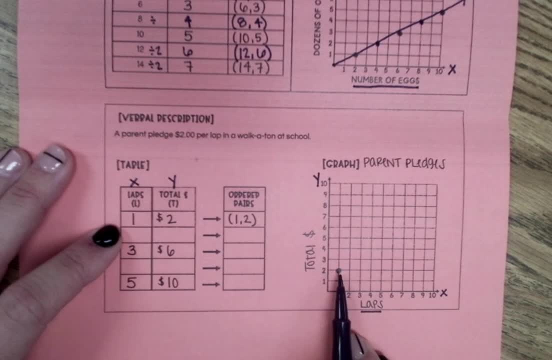 have our ordered pair one comma two And that's our total money. So we're going to go over here at the bottom and you're going to look at the table on your desk And you're going to find out what's the total money that's going to be. Now there's four laps, So that's already been plotted. 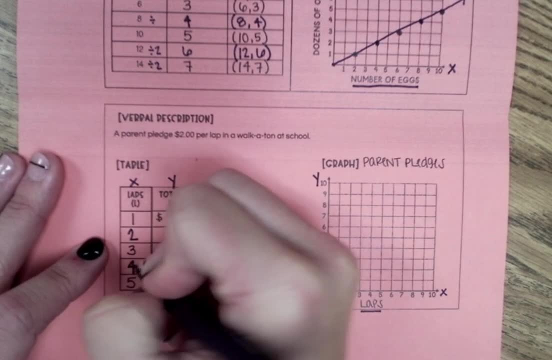 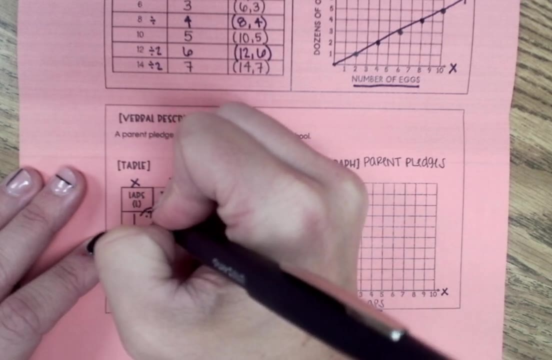 for us. So now we actually get to fill in what we want to for our laps. and I can see I'm going one. I skip a number three, skip a number five. So I'm just going to fill in two and four here. make my 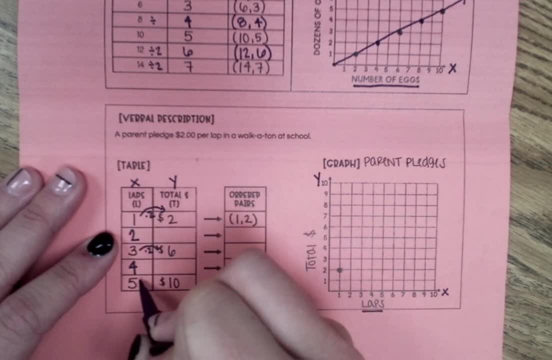 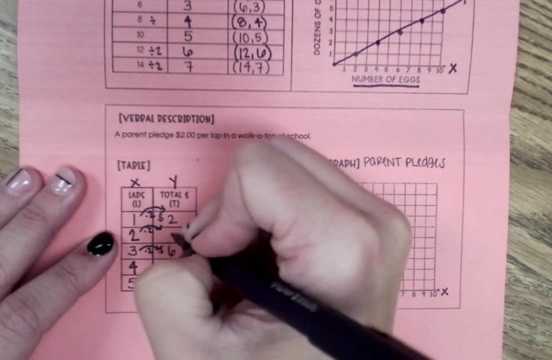 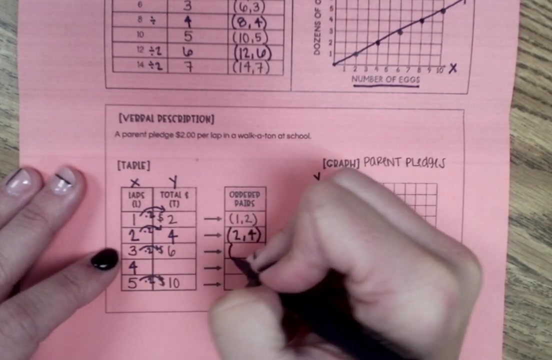 life easier. So I know that from here to here it's getting larger. and I'm multiplying by two. one times two is two, 2 times 2 is 4, so that ordered pair would be 2, 4.. This ordered pair is 3, 6.. 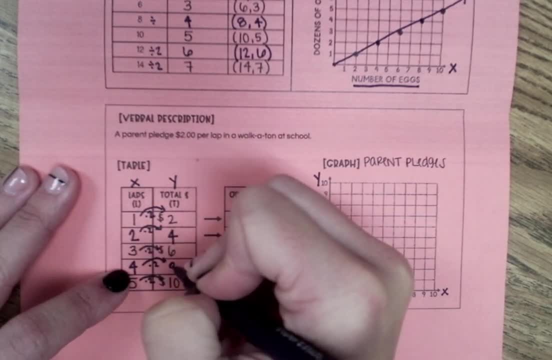 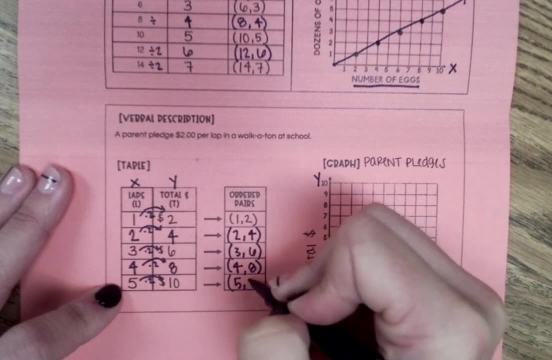 This ordered pair we have to do 4 times 2,, which is 8, so my ordered pair is 4, 8.. And then my last ordered pair is 5, 10.. So now I'm going to plot the rest of my points here. 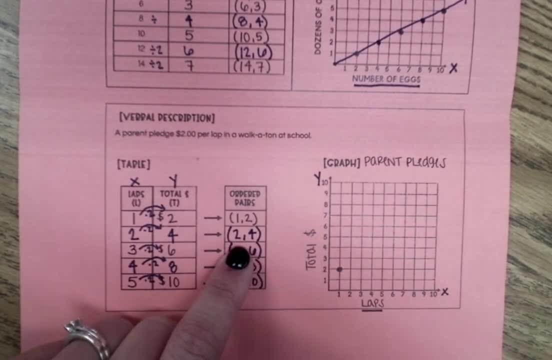 So I see I've already done the 1 over 1, up 2 for that first one. So I'm going to go to my origin and I have 2, 4.. So I'm going to go over 2, because that's my x value, and up 4, because that's my y value. 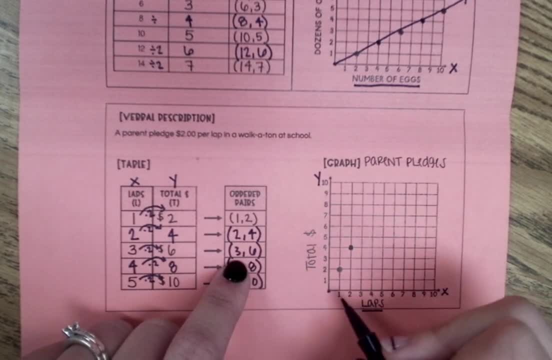 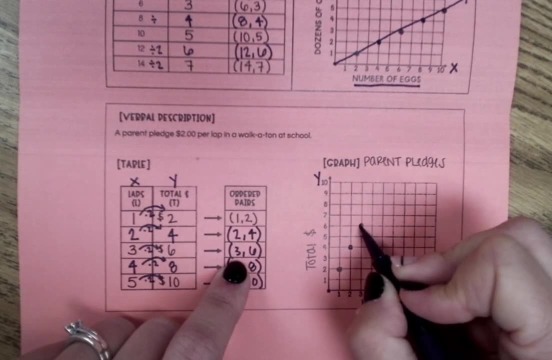 I'm going to plot with a dot. My next point is: ordered pair is 3, 6,, so I'm going to come back to my origin. We go over 3, up 6, plot with a dot. My next point is 4, 8,, so I come back to my origin. 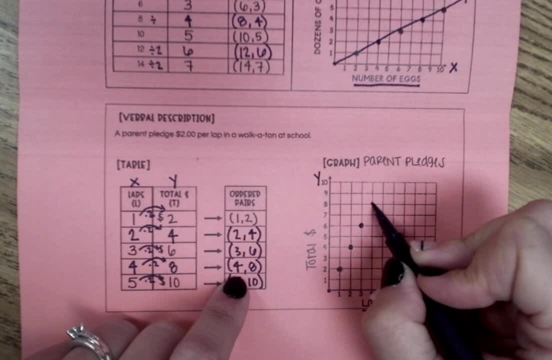 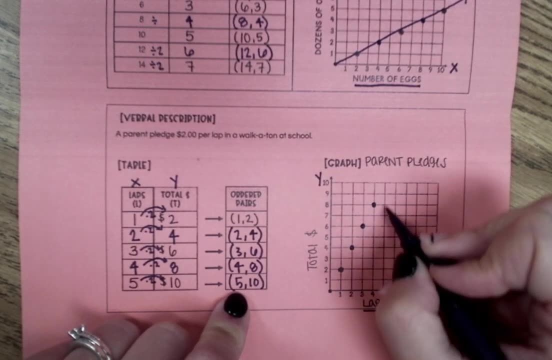 I'm going to go over 4, up 8, plot with a dot, And then my last one is 5, 10, so I'm going to go back to my origin, go over 5, up 10, plot with a dot. 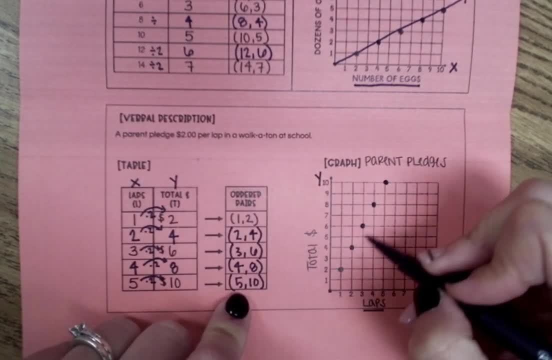 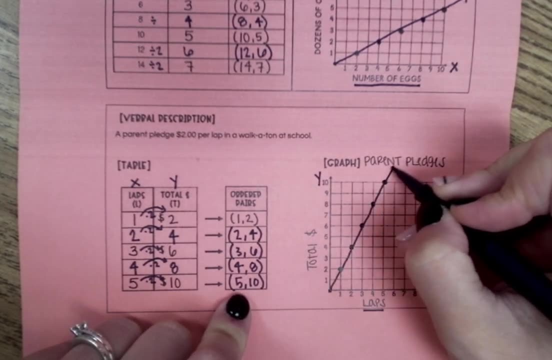 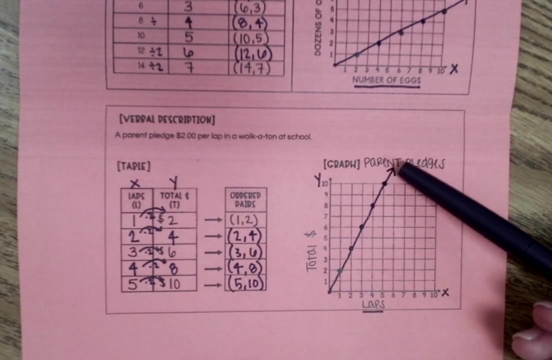 And again, it's going to continue on like this. so depending on how many laps the students do, for how much money the parent is donating, So this as well is just going to continue to go off of that chart. So we're going to connect our dots and we have that little arrow extension to show that that's going to continue on that same trend. 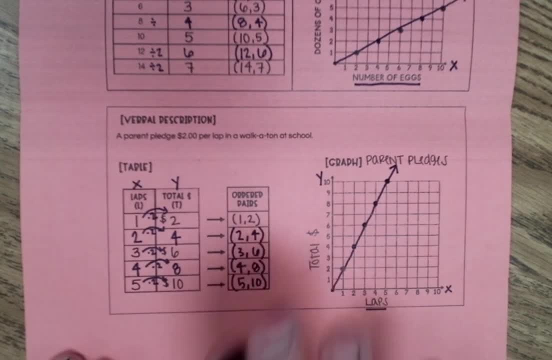 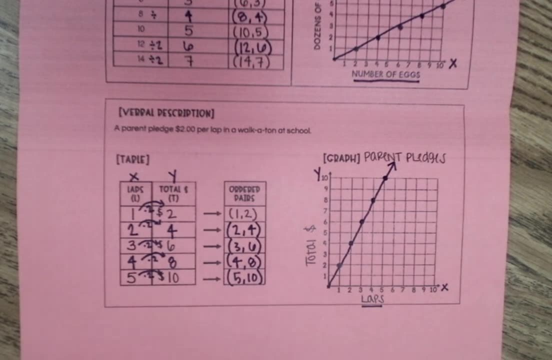 All right, 6th grade. You guys can use this now as an example to look at as you work through the problems. today You will be submitting them on Canvas and when you're finished, you're just going to glue this into your spiral. If you have any questions, please let us know.